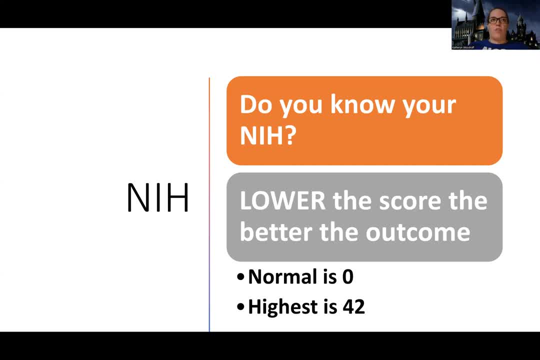 GCS, GCS, GCS absolutely will have test questions where you'll have to score, figure out, like know in depth or be able to like look at that. we could not give you a question. we would have to like make a full video and like it would be lengthy for you to scale or to score someone on this scale for NIH, like it's. 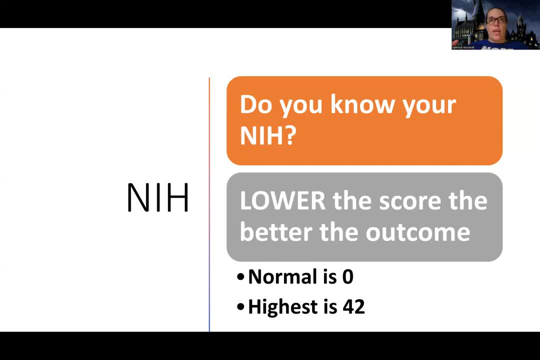 impossible, but what you do. so I'm going to go through the scale so you kind of know what's in it. but I'm not going to go crazy in depth because it's something you're going to have to learn, because, like, I could go over it 15 times and it's just, it's a lot like, it's not something that. 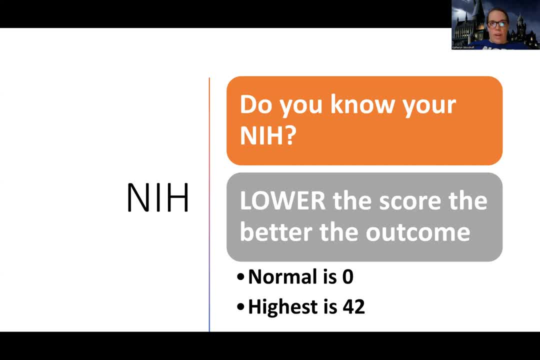 anyone, maybe someone who does it every day has memorized, but most nurses do not have this memorized like literally. we have a handout and anytime I have to do it I have to look at it just to make sure I cover all my bases. but the NIH. what happens is someone comes in it's suspected stroke. 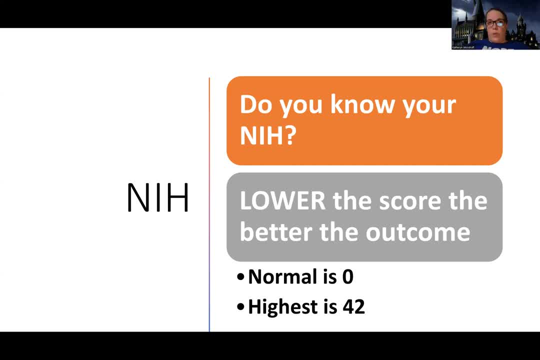 the ER nurse is usually the first one, or even they might do it. you know in the that we usually- my understanding is- we usually start with they do like a mini NIH on the way to the hospital, then in the hospital we do a full NIH and then like, let's say, for 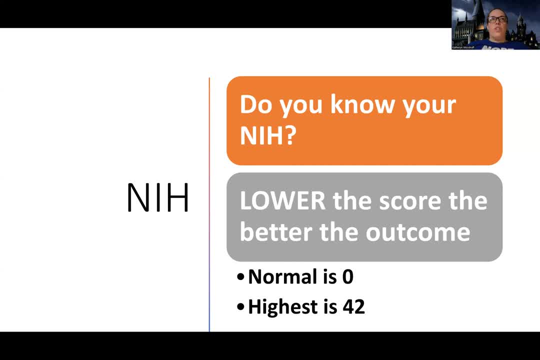 example like the way that I interact with this assessment is if a patient's going straight from the ER to go to like get the clot removed from their brain in interventional radiology, we'll talk about that. if they're going to go there, I'll actually meet the ER nurse in the procedural area. 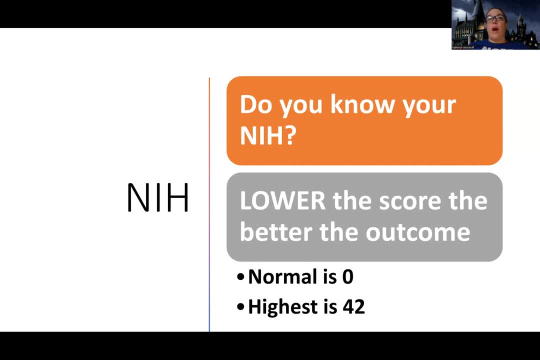 and I will do an assessment on the patient before they put them under that way. I have seen their, because so many things are so different and can change, so this is what my hospital does. I'm not saying every hospital does this, but some hospitals, like I, will actually go down and assess that. 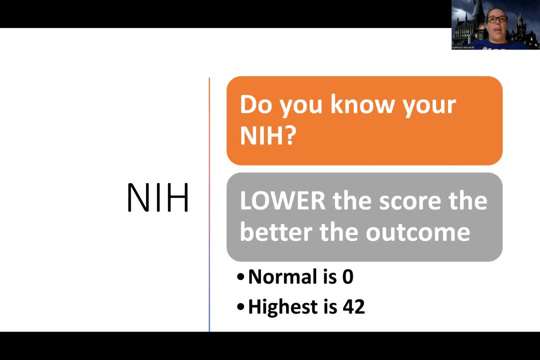 patient before they go and have any intervention done, that way that I can say, hey, here's how they were before and here's how they are now, since I'm going to be the one assuming care of them after that procedure. so the NIH is a longer assessment and it just allows for me to get a more comprehensive. 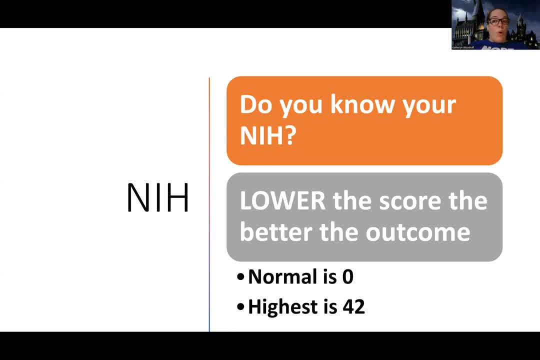 look at how they're doing again. it measures deficits. so the only thing that we would test you over with this is not necessarily like what's the difference between the two, but it's just like what's on this. but you do need to understand what is a sign that an NIH is good, or what's a sign? 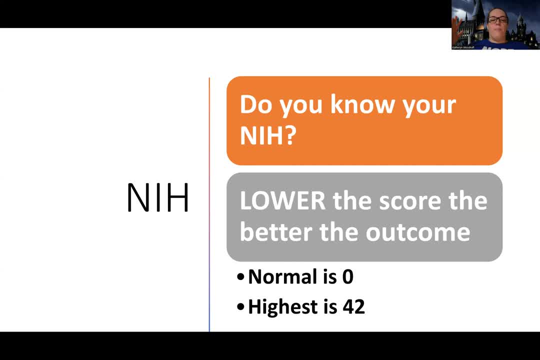 that it's bad. so the normal NIH is what do you call? a normal NIH can range anywhere from a score of 0 to 42. the higher the score, the worse the patient is doing, so the higher the score it's really counting how many deficits the patient has. so we want a low NIH. remember for GCS like. 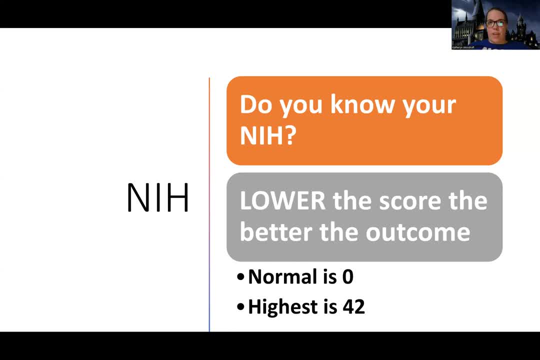 these are both acronyms and you guys can get them mixed up. GCS is level of consciousness. we want a high level of consciousness, we want a low NIH. and so with the NIH again, the lower it is, the less problems the patient's having, the better their. 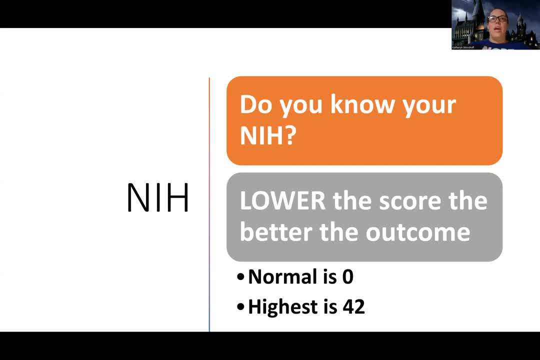 scoring, so we want it to be lower. so we could give you a question and say something about whether the NIH is going up or down. is that a positive sign or a negative sign? so that's all that you'll need to know, or, like you know for some, like if we were talking about treatment after a stroke, how would 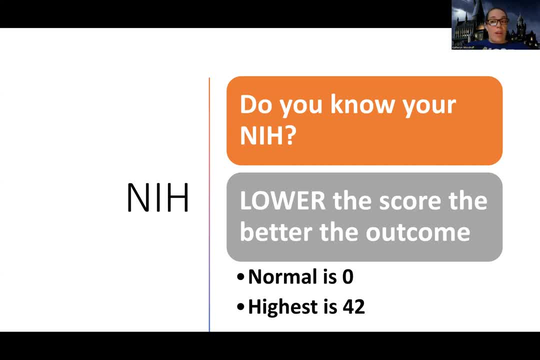 I know a patient's diagnosis is going up or down. is that a positive sign or a negative sign? so it's doing better? if their NIH was improving- and improving I mean going down- then it would be a good sign that the treatment is working. so GCS we want, up high level of consciousness. NIH we want. 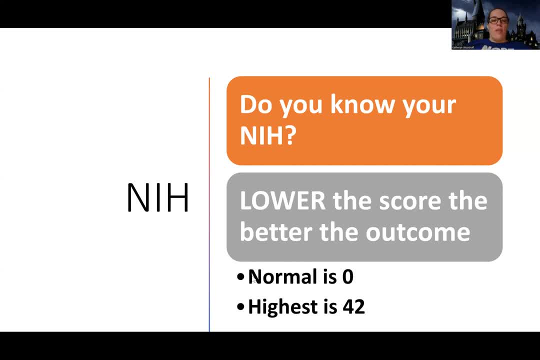 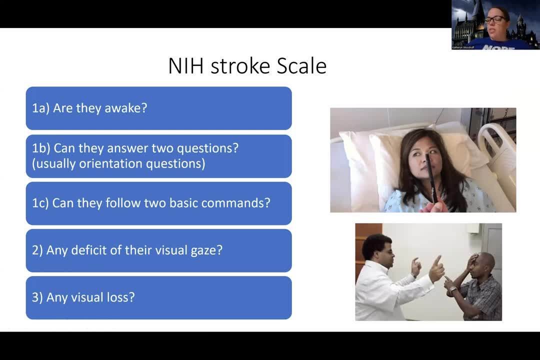 low. we want it down. the lower the score, the less the deficits. so let's talk through this. I'm going to say there's like 13 questions as a part of it, but effectively what is happening with the NIH stroke scale is they're evaluating all the different like cognitive and other functions. 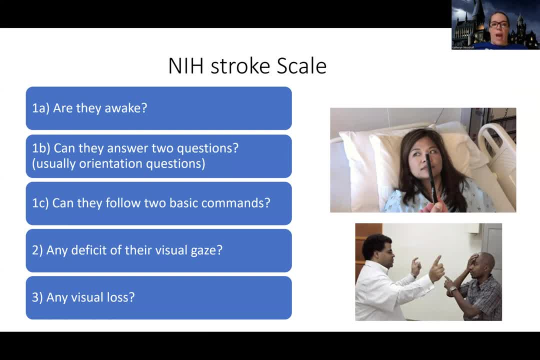 to see how the patient's doing. so one of the first questions we ask is: we do we check orientation and level of consciousness so we see, are they awake? we also asked: see if they can follow commands. can they answer two questions? so and there's like they're like, if you fill this out, like 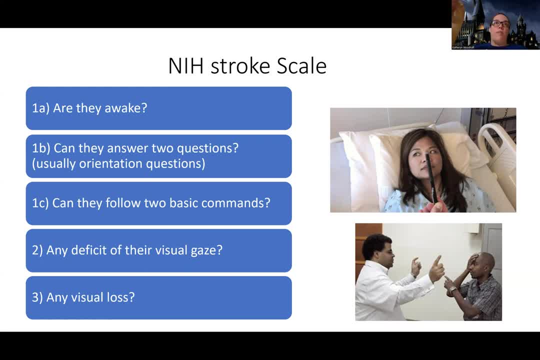 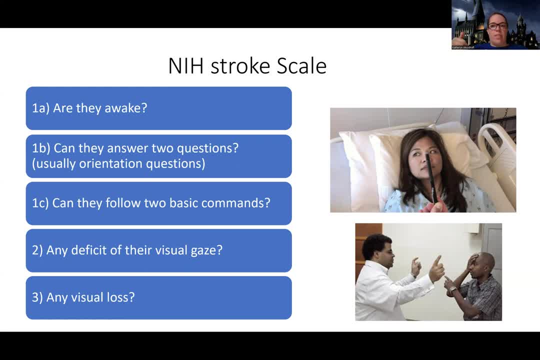 number. so you would see this. I'm not going to go deep into that, but just know like there's a scoring system, just like there is for most of these scales. so are they awake? can they answer two questions? we yeah, sorry, awake. and then for orientation, we usually ask them like what's your? 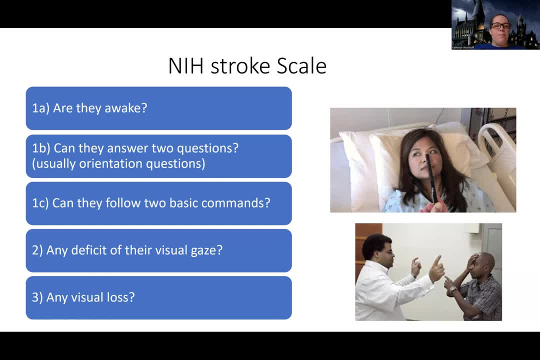 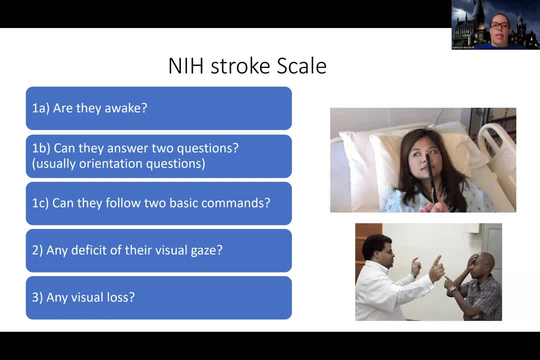 or we got raise your eyebrows, stick out your tongue, something like that- then what? there's going to be some tests that look at visual gaze and that's where they kind of like have you follow the finger across and see if you have any eye movement difficulties, like this lady is here in. 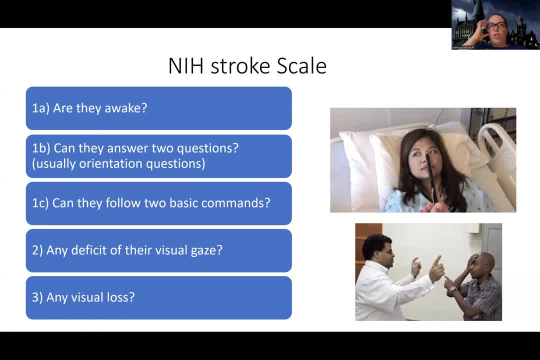 this top picture because you can have decreased motor movement in your eyes after a stroke. they also look for any visual loss. that's where the guy at the bottom is covering this one eye and they literally sit here and go like this and they see, if they can, um, they'll be. like what side? what side am I? um, like you know what's. like you'll do. 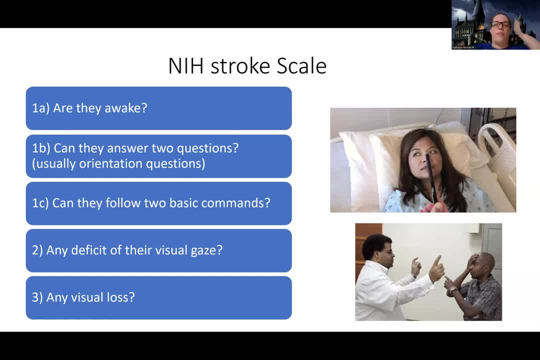 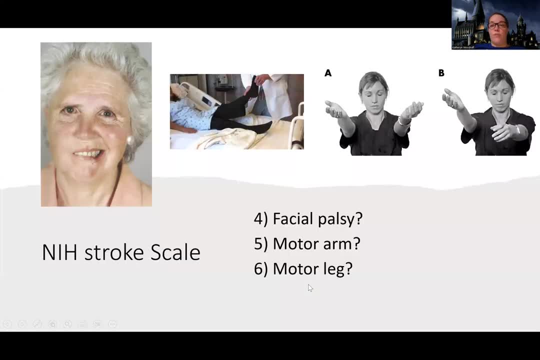 like this and they'll be like, what side am I doing this? and they'll be over here and you have to be able to like, say which side it is. so, anyway, and I can't do it very well to myself, but, um, you get. you get the point. there is videos too, if you want to watch and learn about this. but again, I promise. 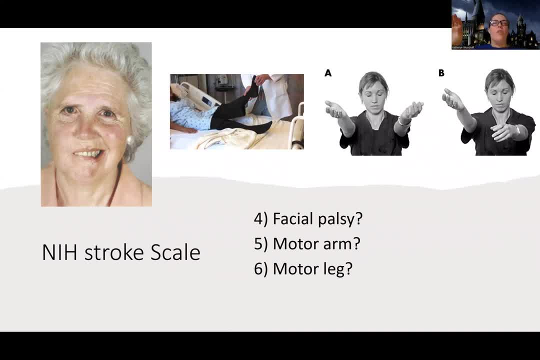 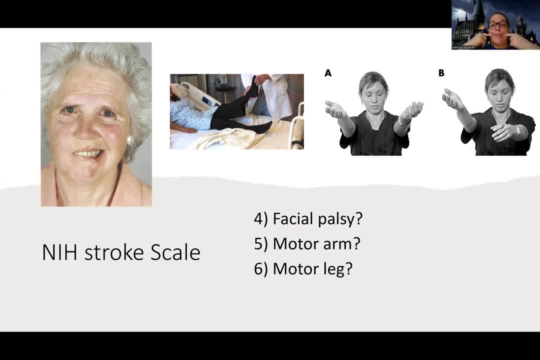 and then raise their eyebrows too, because they can have a droop in their eyebrows. they can also have a droop here. it's called the nasolabial folds. fancy words, but we look for any sort of decrease or deficit. but you can see her in this picture how she has a, a droop on one side then 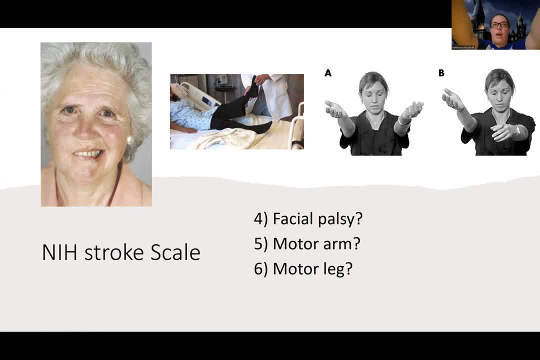 the motor, the arm. that's where we stick the arms out and then see if one drifts. we have them hold their arms up for 10 seconds and then see if there's a drift, and then we usually have them do both arms at the same time. 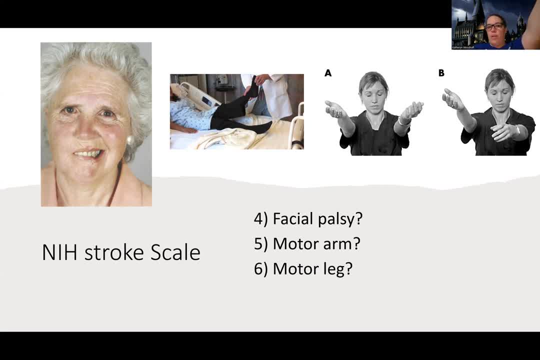 no, never mind. no, usually I'm thinking about it just one arm at a time. can you hold it up for 10 seconds for the legs? we have them hold up for five seconds, one at a time. definitely don't ask them to hold both their legs at the time. maybe with arm drift we do have them at the same time. I can't. 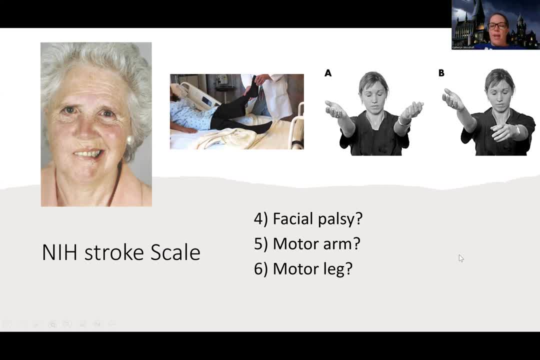 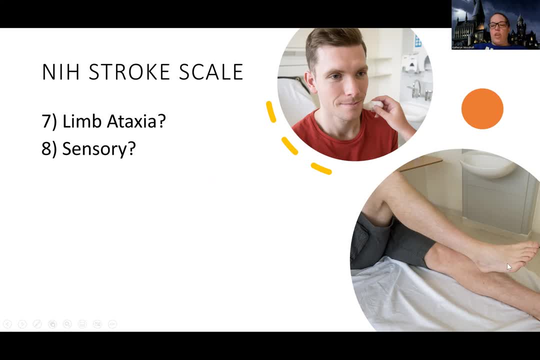 remember now I'm having- I'm having a moment, maybe I'm having a neurological deficit myself. let me do limb ataxia, and I'm not going to try to show you this one. you effectively take your heel and rub it up and down on your shin. 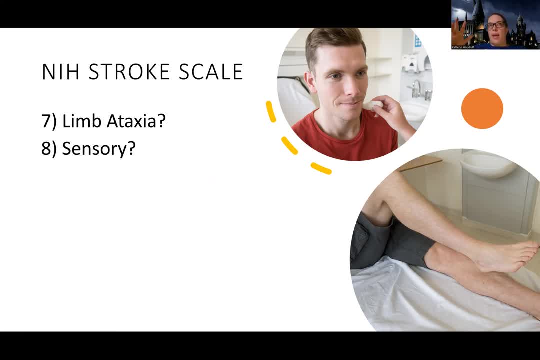 and this is just to see ataxia kind of. I always remember ataxia is like you need a taxi to get around. it's kind of like you, it's like a abnormal gait, or what do you call it- where your balance is off. so it's really just seeing if you can run your heel up and down your shin. 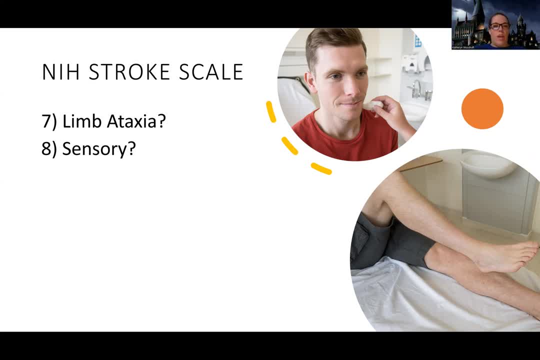 with coordination. so kind of think of it, looking at coordination, then sensory. this is where they they use a variety of types of pressure. they might use soft pressure or harder pressure and they're pretty much seeing side to side like they might touch and say, like does one? 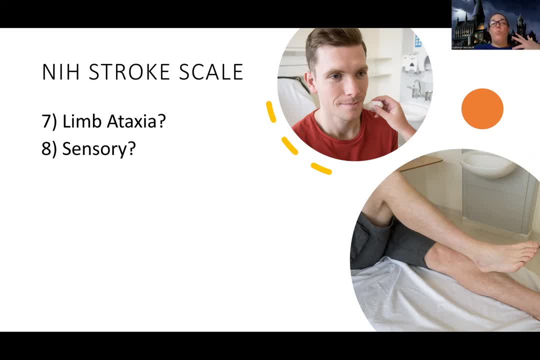 feel sharper than the other, one or just one? do you feel one side more than the other? and they start your face and make their way down to your, your arms, your legs, and see if you can feel better or differently on one side than the other. then they start getting into some of the cognition. 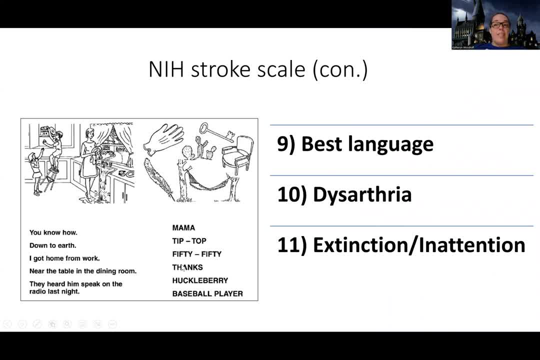 and other stuff. so they'll do things like check your language. so this is literally the thing that you will have, and everyone has the same one- and they will check your language. they'll ask you to read these sentences. they'll say: you know how, down to earth, I got you down to earth, down to earth. 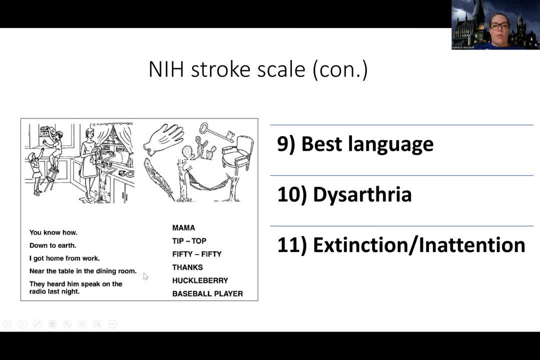 I got home from work near the table in the dining room, so they'll have you read. they'll also have you look at the this picture and have you describe it like. they'll say what's happening in this picture and they'll see if you can talk about it and how fluent your speech is around it. they'll 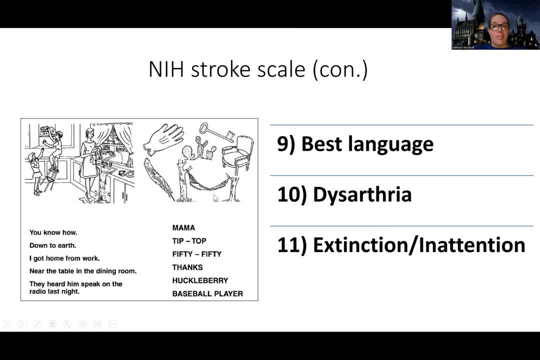 also have. you look at this, these objects, and see if you can identify them. there's something called agnosia that can happen after a stroke, where you can look at an object but not be able to say it. you could be holding your phone and not know the word for phone. so they're seeing if you can. 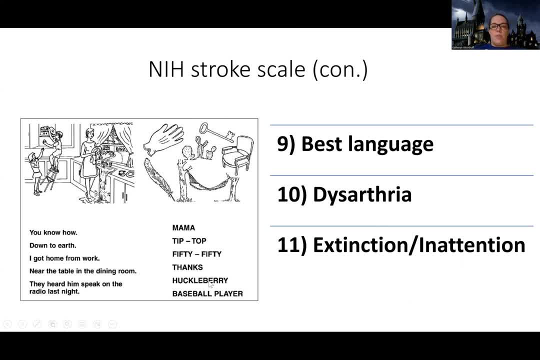 identify these objects. and then this is this one with the words on the right hand side is what we call the dysarthria test, and a dysarthria test is looking for abnormalities in articulation. so there's speech, like my ability to sit here and just communicate, but there's also articulation. 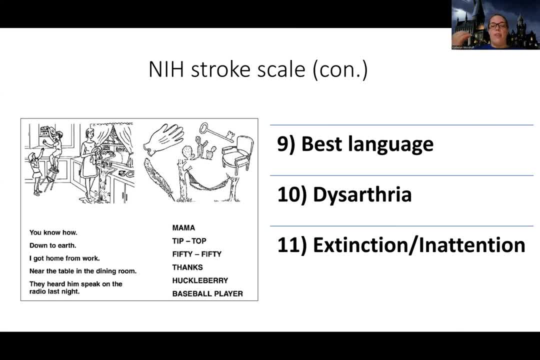 where you can hear all the words that I am saying, so like if you think these were. these words require more enunciation. so with dysarthria, someone's gonna it's gonna be really hard to understand the words they say. when someone has dysarthria, it's actually because of the stroke. 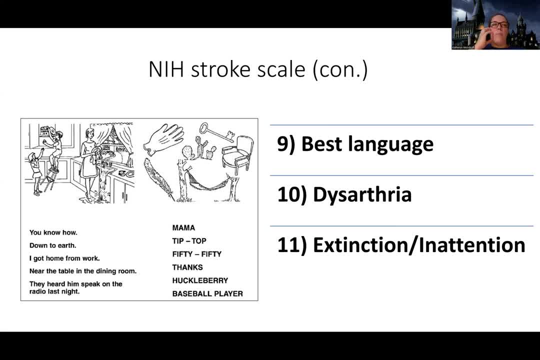 like it, it, um, it weakens their jaw or the muscles in their mouth or in their throat, and so it leads them. it's harder for them to talk, they can't really articulate well and it's hard to understand them, um. so for this one it's like mama tip top 50, 50 and someone who has um dysarthria. I'm not, I'm not. 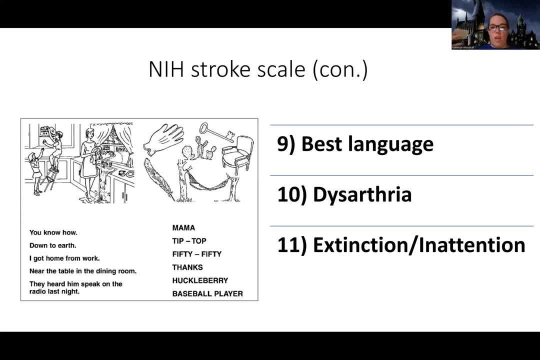 going to do this. well, but, yeah, like you can't really understand them, it's going to be like they can't really, um, they don't have the muscle strength to really articulate those words. um, then, extinction or inattention, um, that's where they're going to like usually have you close your eyes and they're going to tap on one leg or 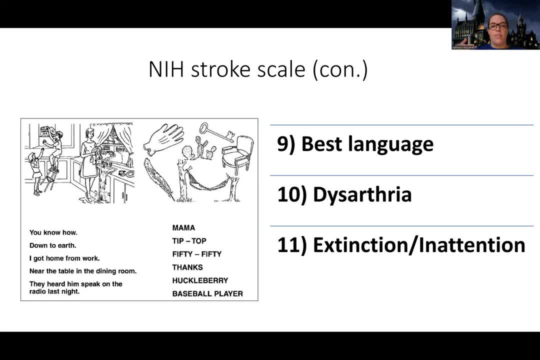 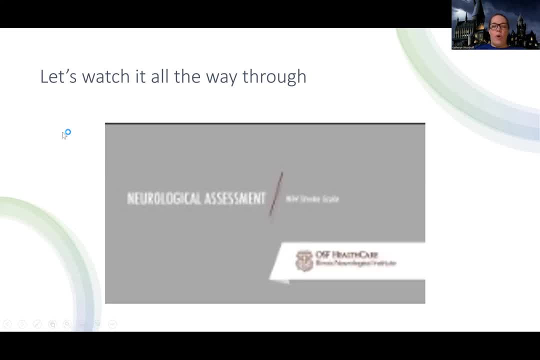 the other and see if you are giving attention to both or you can feel both of them, because sometimes people have one-sided neglect or they cannot feel on one side, um. so I found this like online video, um, and it's okay. they they do it with a normal person, so it's not like they're. 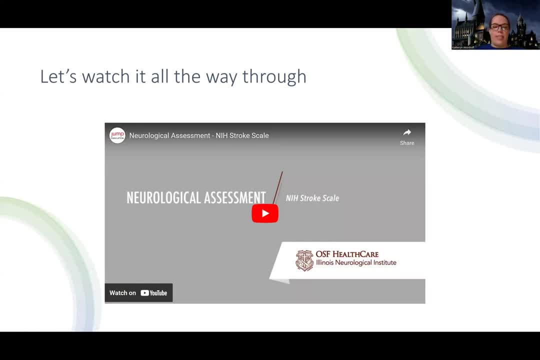 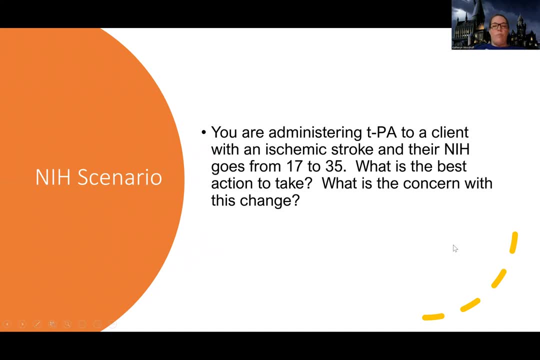 so it's a little hard to say, but if you wanted to see more about um, what it looks like, definitely you can watch it all the way through. all right, oh, I have a scenario before we end, since you are administering tpa, which I know. you guys, we haven't talked about tpa yet, but let's act like. 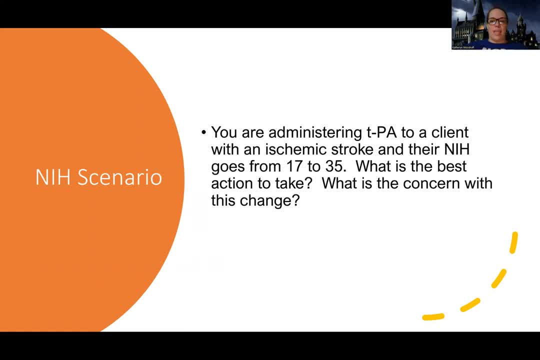 you know what it is. so we're administering a treatment for stroke to a client with an ischemic stroke. their nih goes from 17 to 35. what is the back best action to take? what is the concern with this change? so we have to think about: okay, what's the issue here? I'm giving a treatment to make a